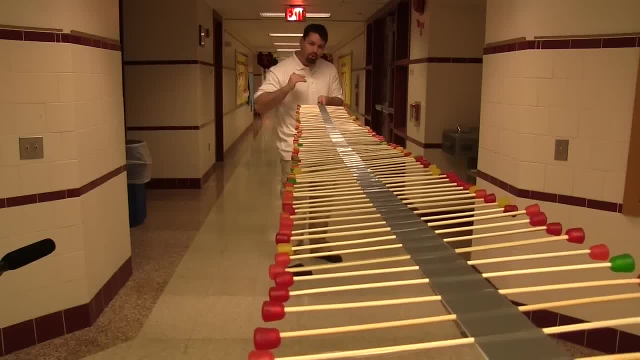 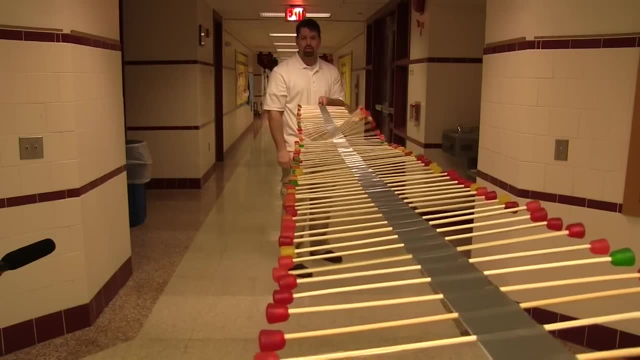 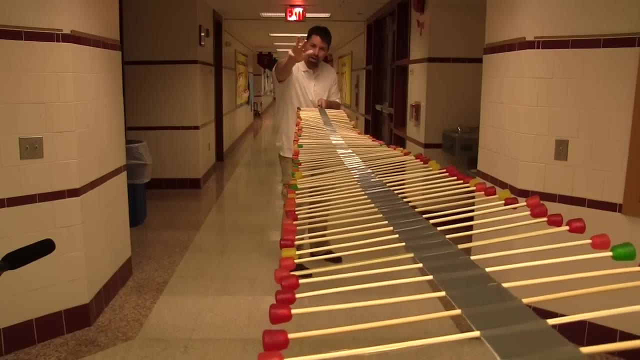 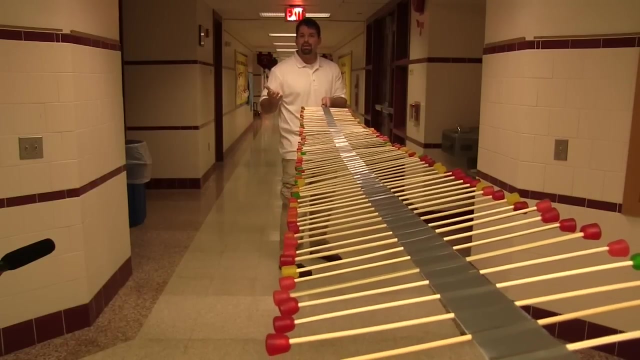 And when I do that, I want you to watch that energy move down the machine from one end back to the other. Watch, Did you see the energy move down the machine and then back, and then back down the machine and back toward me. Remember, sound and light are both energy and they travel in waves, a lot like this. 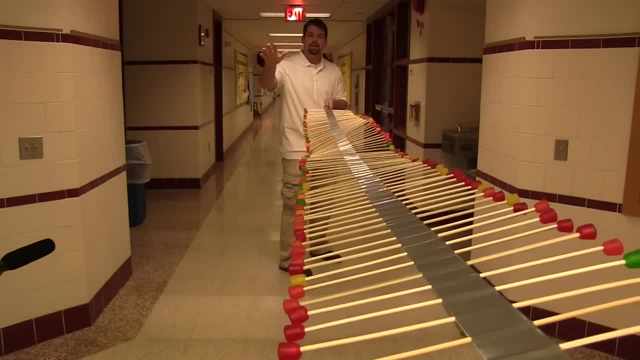 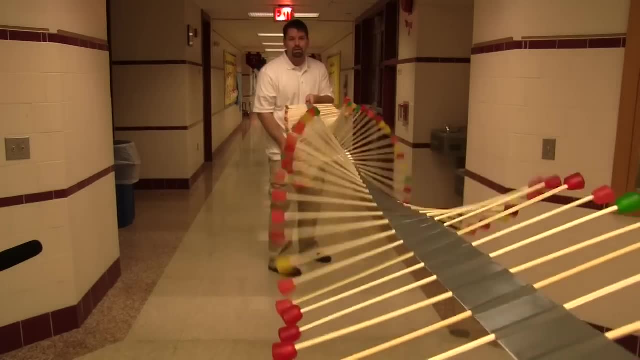 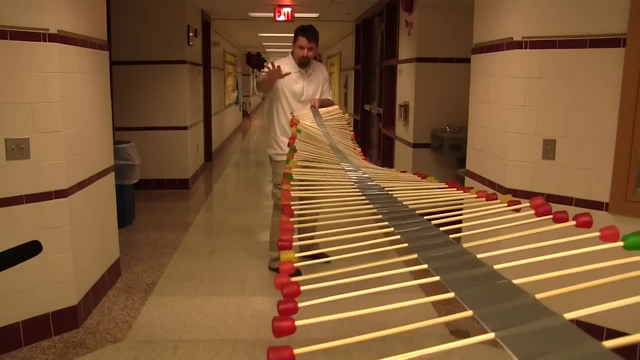 Sound energy and light energy are traveling in waves. Let us see what happens when we add more energy to our wave machine. We get a nice clean, crisp wave that travels down the machine and back and down, and back and down and back The candy wave machine. 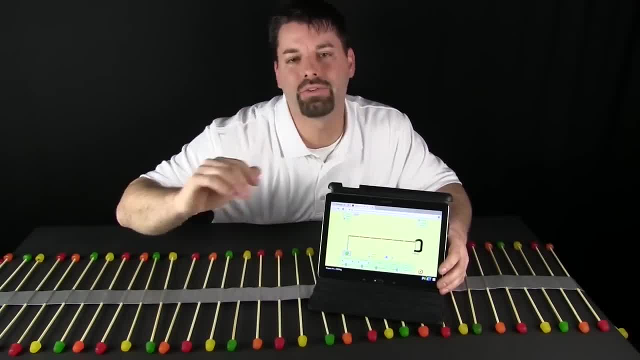 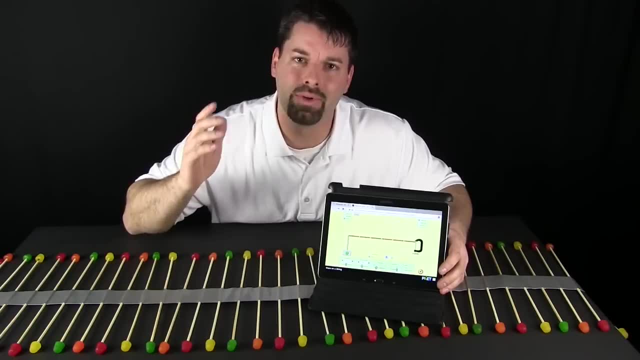 It was so cool to see how that wave energy traveled down that wave machine. But if you wanted to explore waves on your own, there is a great simulation put out by the people from PhET And we are going to zoom in and explore it a little bit to see what that does. 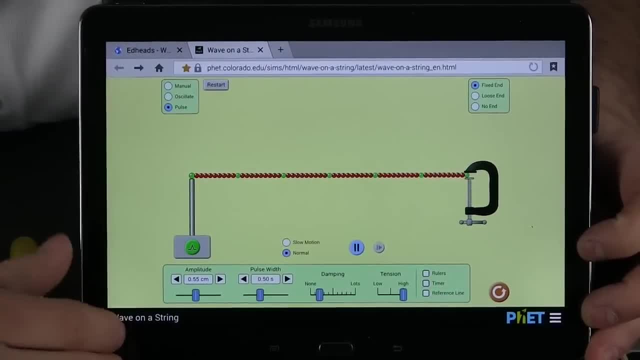 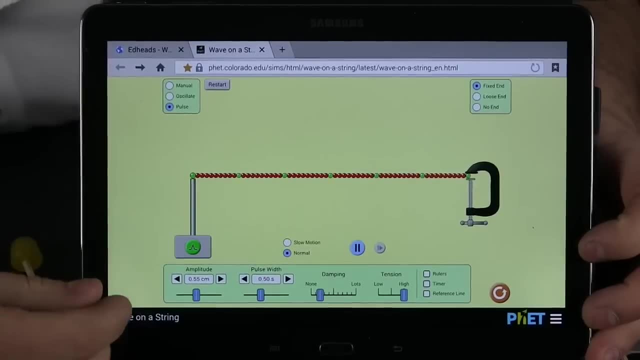 The simulation is called Wave on a String, So let us take a look and see what it can do, Explore it. Well, I see a wave machine that looks a lot like our wave machine. It is stretched out And just like we put some energy in our wave machine to see that wave travel. 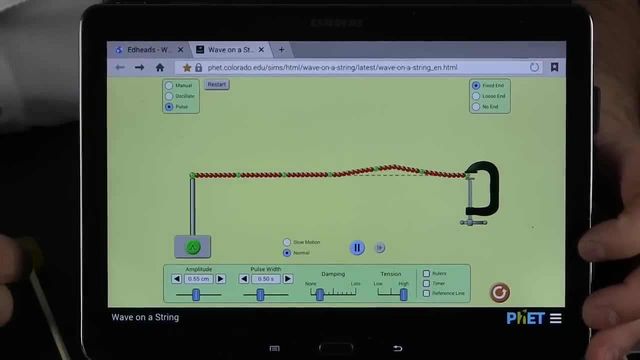 let us put some energy into this wave machine And there the wave is. You can see it travel down from one end and back to the other. Let us do it one more time. What happens? if I make that energy bigger, It will produce more energy. 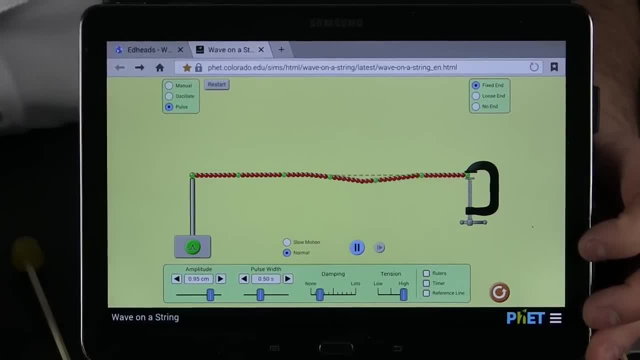 I can turn up a little dial here and make my wave bigger. I can turn it up all the way and put more energy into it And you can see my wave gets bigger. The other thing we can do if we wanted these waves to come automatically is we can hit this button up here. 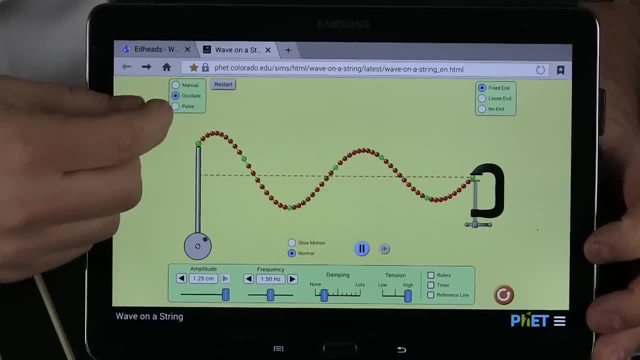 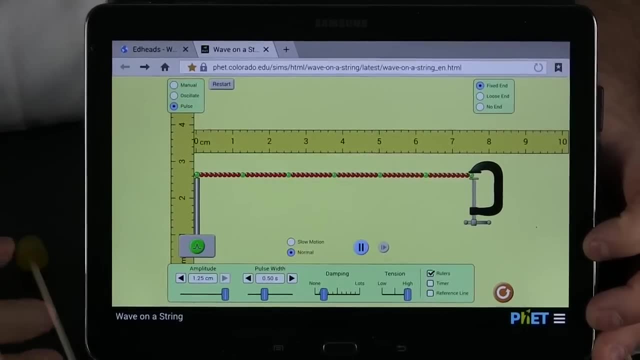 And the machine makes the waves come automatically. We can also hit this button up here if we wanted to collect some data and really measure things. Rulers, come onto the screen. There is so much that this simulation can do. You can explore it on your own.